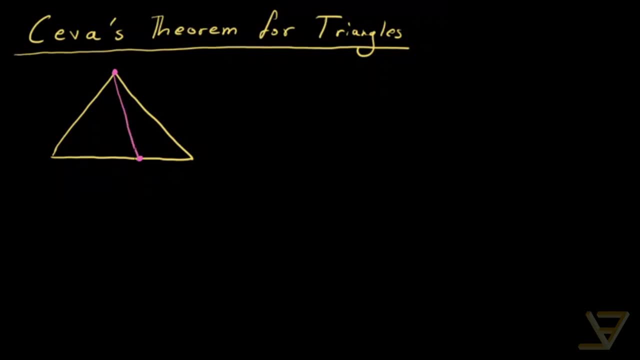 triangle And we then draw this pink line segment that you can see here. So this segment is called a Chevian, And what Cheva's theorem talks about is when you have a triangle like this and you are talking about Chevians from all three vertices being concurrent at. 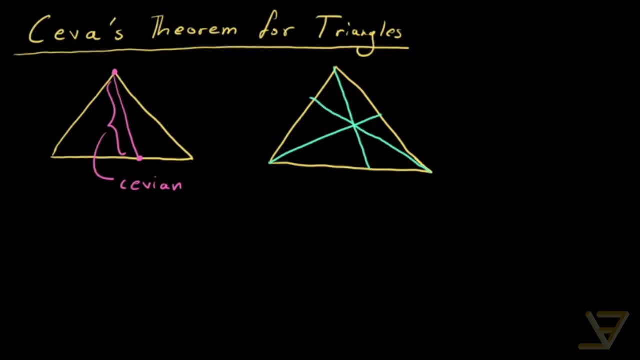 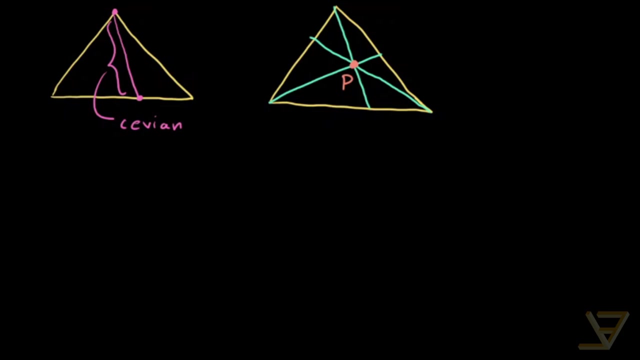 some point in the interior of the triangle, like this orange point here. Let's call it P. So we want to characterize exactly when that happens. and it's going to be two directions to the theorem. In the first direction, suppose, let's call these points A up here, B down here. 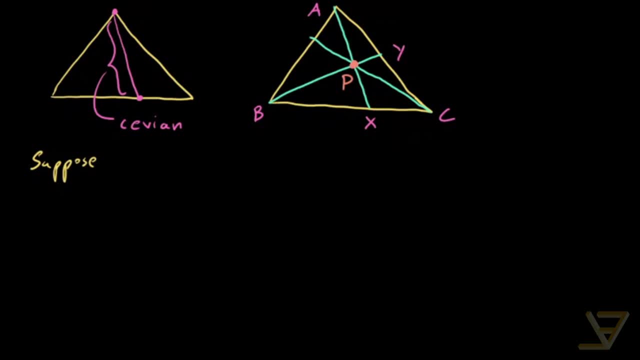 C down here, X here, Y here and Z here, And suppose AX, BY and CZ are concurrent at P. So in this direction we're assuming that there is a point of concurrency. In the other direction we're going to prove that there is a. 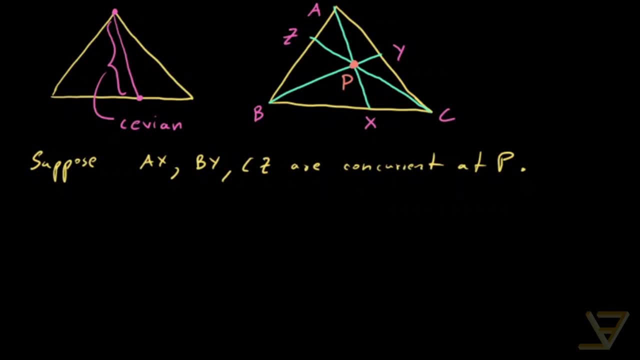 point of concurrency. So let's see what criterion we end up with. We're going to be using a certain amazing algebraic fact that if you have the ratios A over B equals to C over D, then A over B and C over D also equals to A minus C over B minus D and A plus C over B plus D, assuming 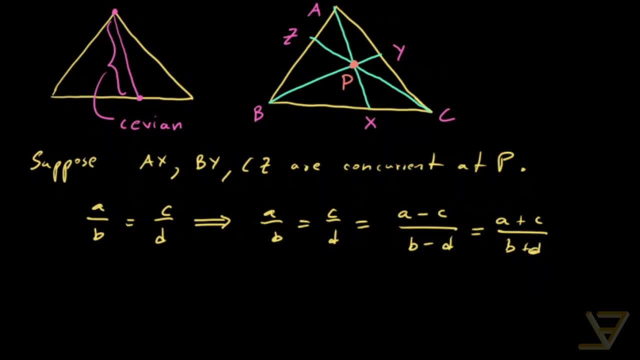 these denominators don't equal to zero And you can prove this just by clearing the denominators- I believe it's called cross multiplication- and just expanding out. So when we use this, we get the following result: Because BX and triangle, ABX and ACX share a height, this height- here I'm just going to get your- 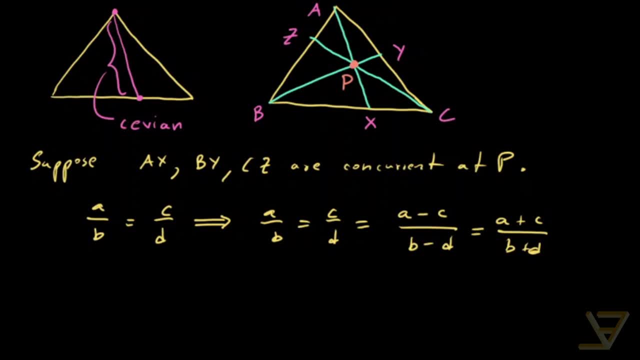 ​ included in to the diagram so we can erase it so it doesn't get too messy. We find that BX over XC is equal to the area of ABX over the area of ACX and that is equal to area is of PBX over the area of ABX. 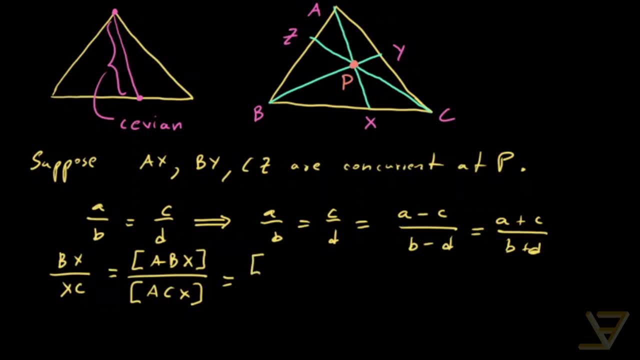 ​ And the area of ABX. ​ And the area of ACX. ​ ​ ​ ​ ​ ​ ​ ​ ​ ​ of PCX because there's a common height for those two triangles here. So what we can do is subtract these numerators to get ABX minus PBX over ACX minus PCX and 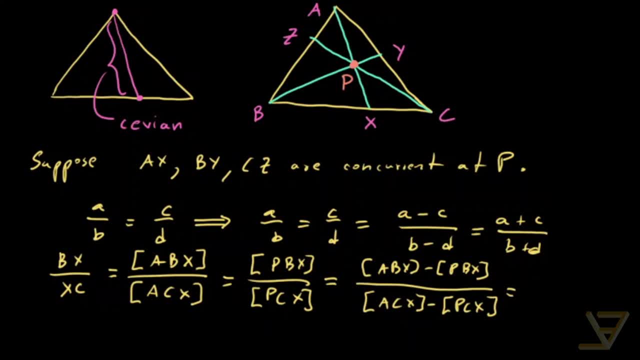 what we find is that these are equal to this triangle here, so that's triangle ABP over this triangle here, so it's triangle area of triangle ACP. So that's our first result, and we can make analogous equations. So what we get then is: 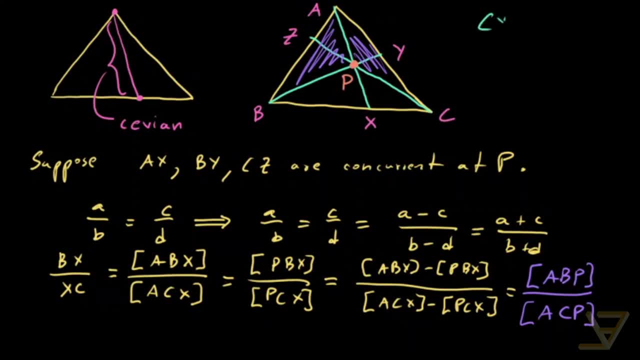 a z over zB is equal to The area of Cета. It's AP divided by the area of CBP. and now what we're going to do is we're just going to multiply all these equations together. so we've got this: equals to this. so that's our first equation. 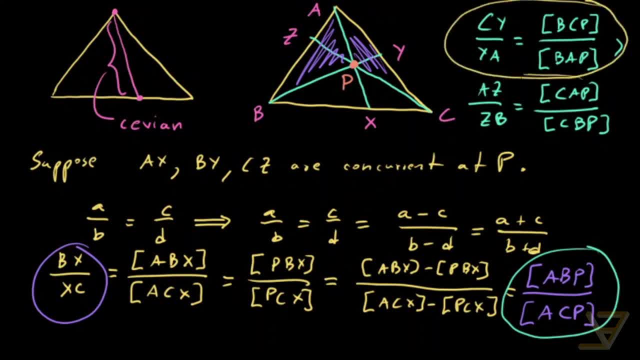 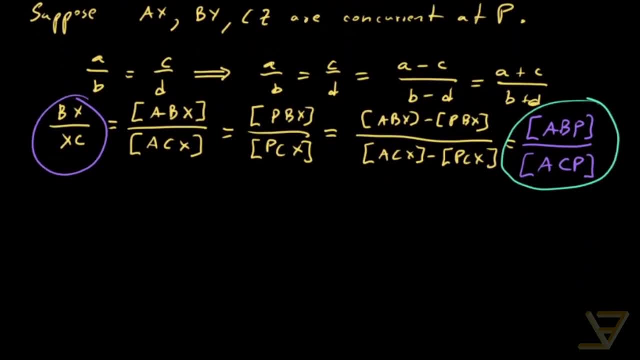 we've got this over here, that's our second equation, and this over here, that's our third equation. so let's multiply it all out. if we multiply it all out, we get that bx over XC times, CY over YA times, AZ over ZB is equal to a BP over a CB. 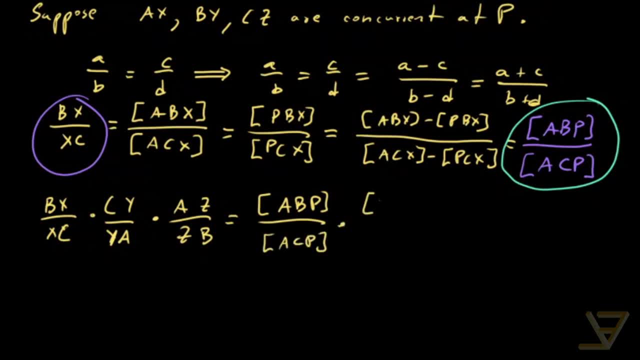 BCP times BCP over BAP, times CAP over CBP. So let's see what cancellations we get here. We get that ABP and BAP cancel out, We get that BCP and CPB cancel out, And we get that CAP and ACP cancel out. 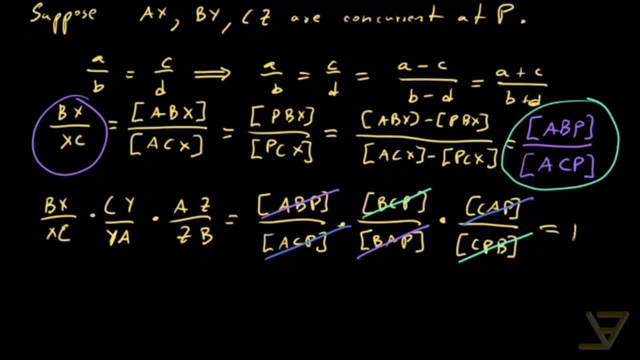 So in the end, we're just left with one. That's a pretty amazing criteria that this quantity over here, this product of ratios, is equal to one. Now let's go in the other direction, Because this is Chavas theorem that we just proved. 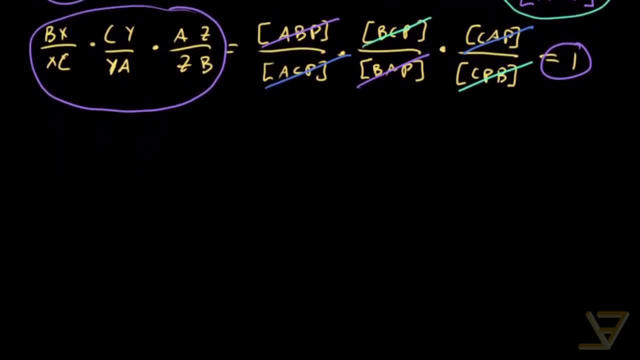 But the converse of Chavas theorem also works as well. So suppose BX over XC times, CY over YA times, AZ over ZB is equal to one. What we're going to be doing Is using a technique called phantom points, Which sounds ridiculous. 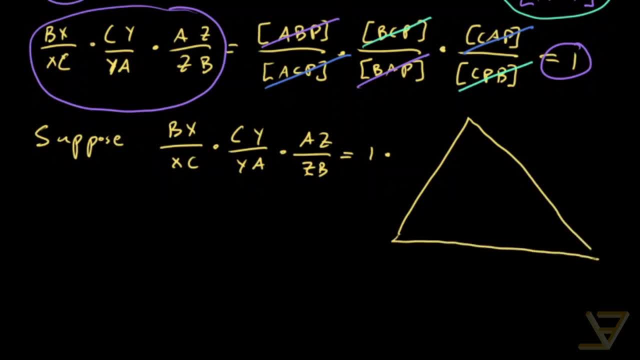 But it's actually quite useful, especially in Olympia geometry. So suppose we have A triangle ABC And suppose that we draw the chevion out of B which goes to Y And the chevion that goes out of C which goes to Z. 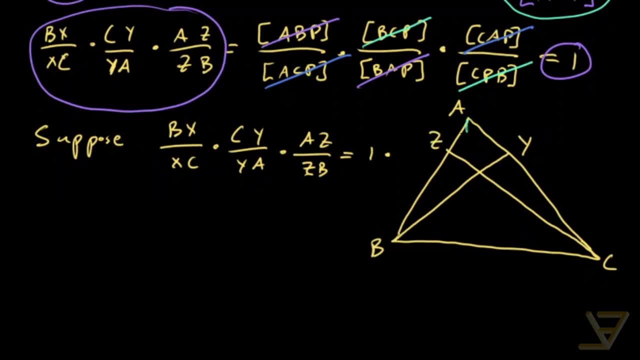 Okay, And we don't know if the chevion out of A is going to go through this point, But we're going to show that it does. So let's say it's just some generic chevion like this that goes to X here. 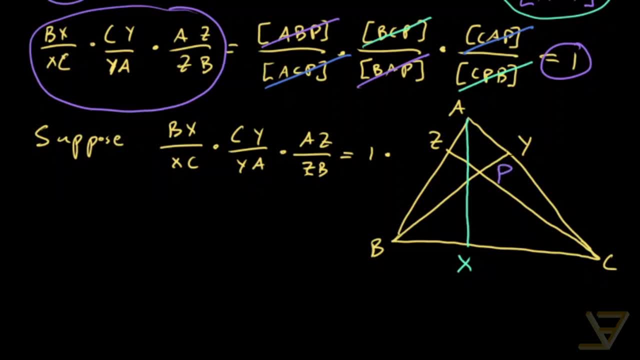 And suppose we draw the chevion that does go through P and through A, And we're going to say that hits BC at X prime. Okay, So what we want is that X equals to X prime, And that's what we're going to show. 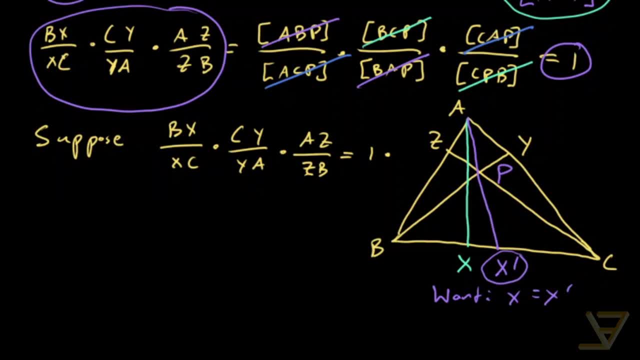 The phantom point is this: X prime. So let's show that X equals to X prime By Cheva, And this is one of those cases where one direction of a theorem proves its own converse. So by Cheva, since AX prime does go through the concurrency point. 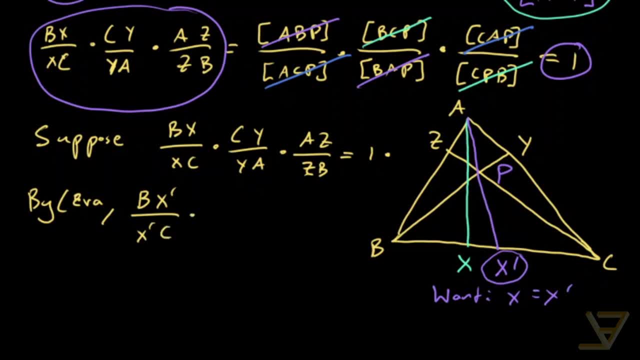 We get that BX prime over X prime CY. Okay, So we're going to say that X prime over X prime, C times C prime over YA, times AZ over ZB equals to 1.. And now what we're going to do is we're going to take the assumption here: 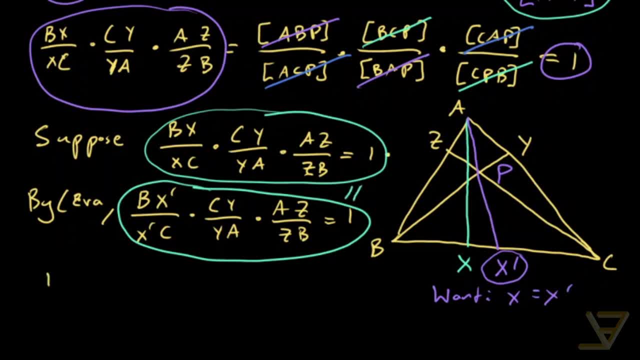 And we're going to take our derived formula here And we're going to set them equal to each other. So what we end up getting is that BX over XC is equal to BX prime over X prime C. Okay, But we also know something else. 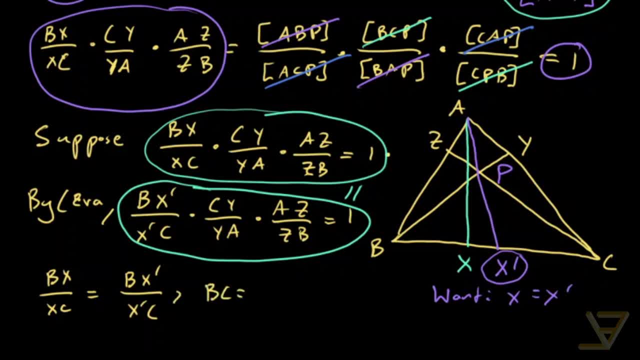 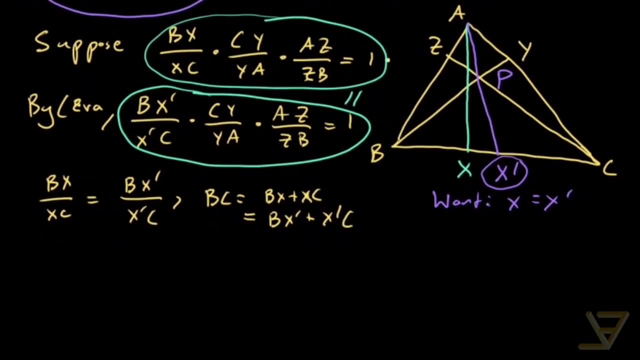 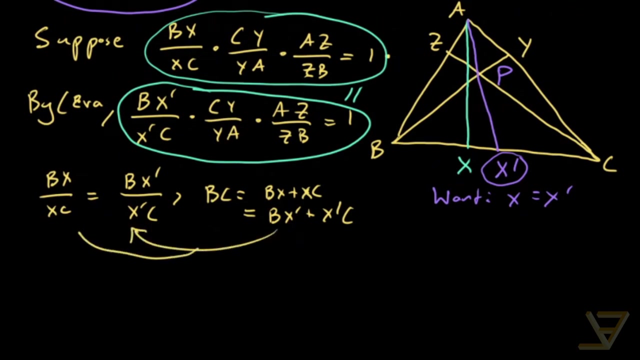 We know that BC is equal to BX plus XC, And we know that that's also equal to BX prime plus XC prime. Sorry, It should be X prime C. So what that tells us is that we can make a substitution from here into here and into here.